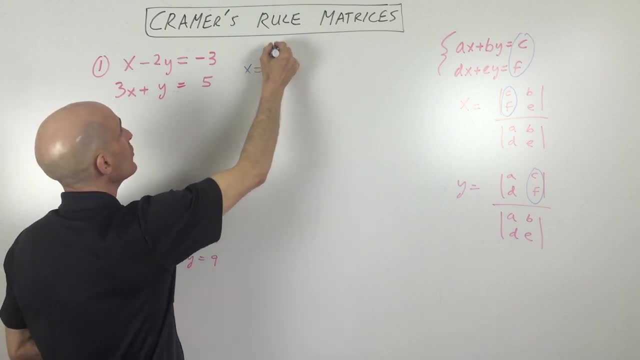 So what I'm going to do is I'm going to set up Kramer's rule. We've got x equals the determinant of. okay, do the numerator and denominator, and I'll do the same thing for y. So I'll show you kind of how we work through this.